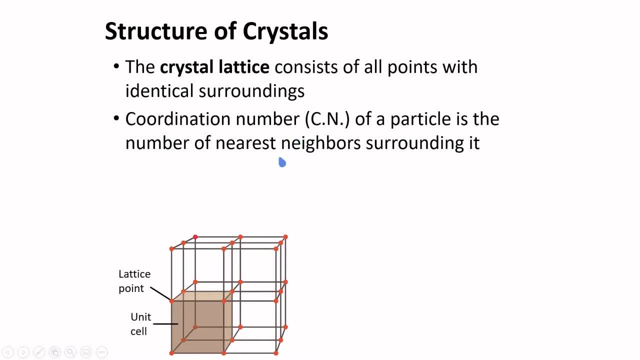 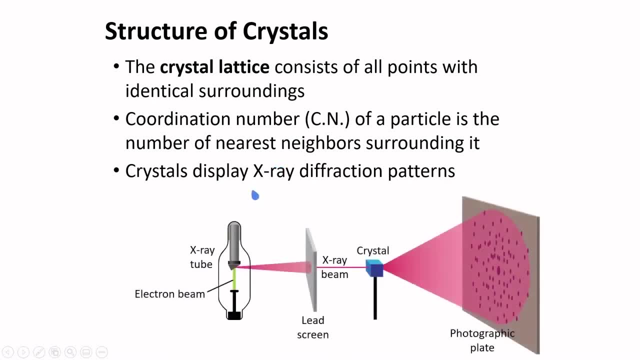 a particle is the number of nearest neighbors surrounding it. Crystals display x-ray diffraction patterns. As x-rays pass through crystals, the beam is diffracted to form a pattern. This pattern allows for the analysis of the properties of the crystal lattice. 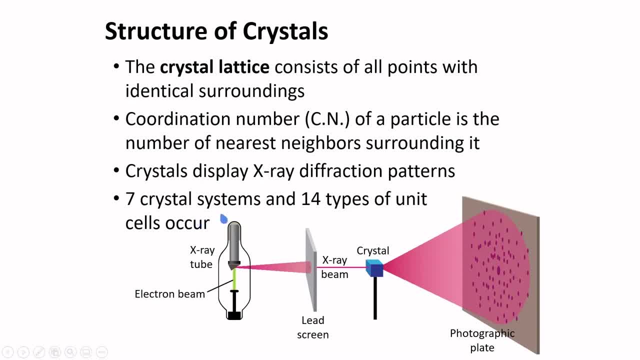 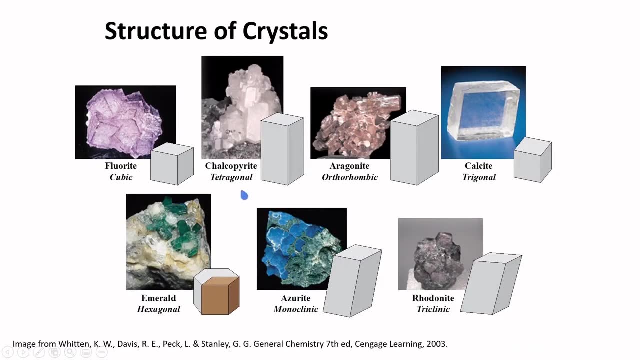 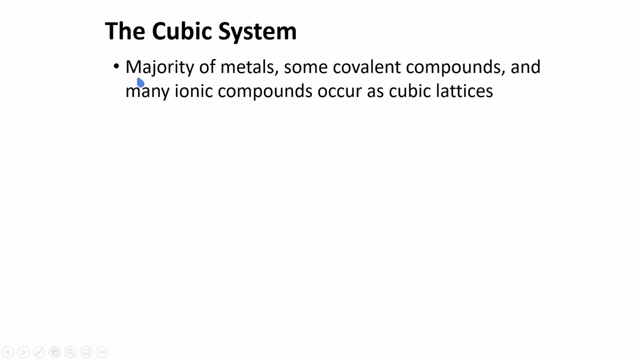 Studies indicate that seven crystal systems and 14 types of unit cells occur. These crystal systems are the cubic, the trigonal, orthorhombic, trigonal, hexagonal, monoclinic and triclinic. of the seven crystal systems, i will mainly talk about the cubic system. 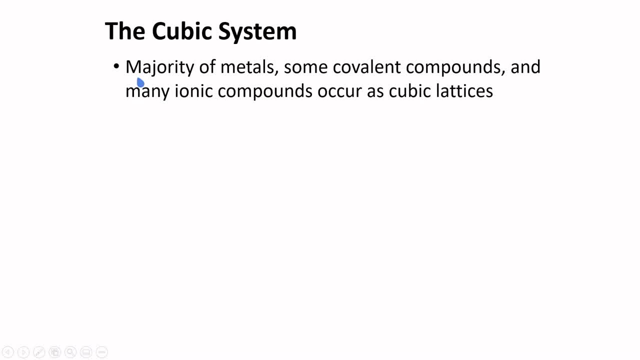 the majority of metals, some covalent compounds and many ionic compounds occur as cubic lattices. there are three types of cubic lattices. the first one is simple, or primitive, cubic cell. here the centers of eight identical particles form the corner of a cube. assuming there is only one type of particle, the coordination number here is six. 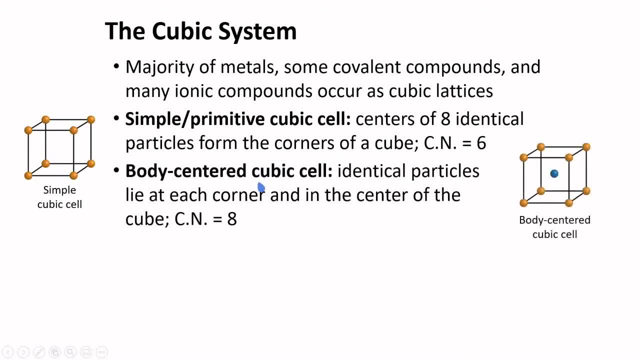 the next type is body centered cubic cell, wherein identical particles lie at each corner and in the center of the cube, the coordination number for a system with one type of particle is eight, and in the center of the cube, the coordination number for a system with one type of particle. 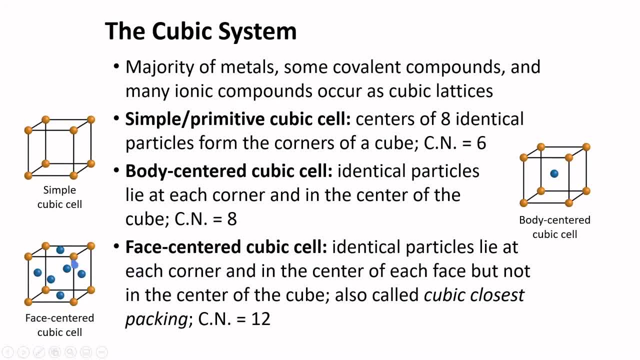 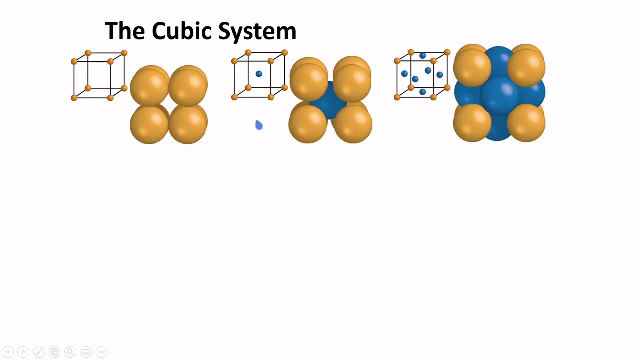 is nine. face centered cubic cell has identical particles lying at each corner and in the center of each face, but not in the center of the cube. this is also called cubic closest packing. coordination number in this case is 12.. 2.302 Eternal particles: here again are the particles packed according to the three types of cubic cells. 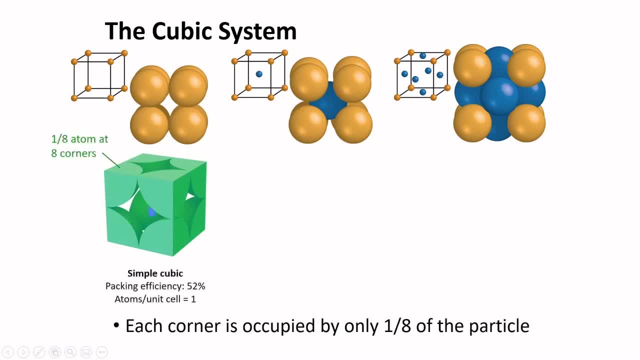 in principle, only portions of particles positioned at the corners and the sides form part of the unit cell will result to one atom per unit cell. simple cubic cells are not very efficient in terms of packing. it only has 52% packing efficiency. if we are to determine the radius of the particle, we can just take the length of one side. 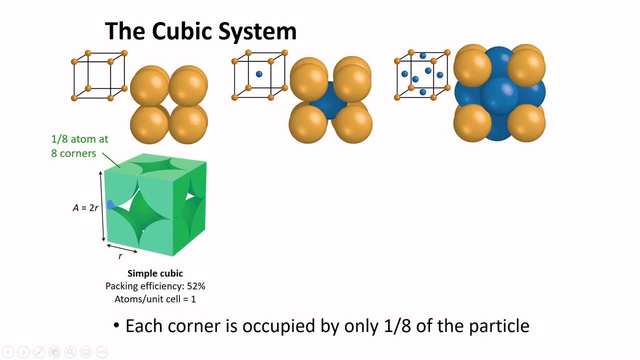 taking note that each side is 2r or twice the radius. the radius can be easily calculated for body centered cubic. the packing efficiency increase to 68% if we take the one whole atom in the middle and the 1 eighth of the particle on its side. 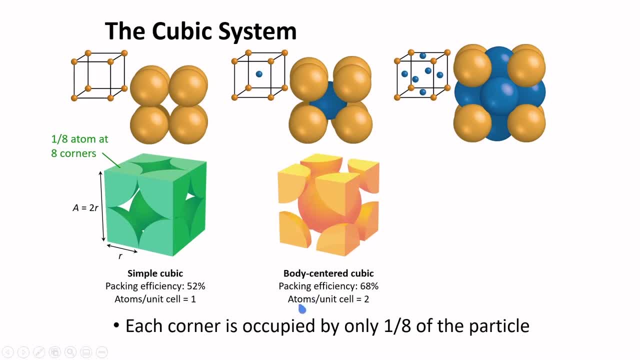 there will be two atoms per unit cell. to determine the radius of the particle we need to use Pythagorean theorem. if the length of the side is known, then B can be determined. B squared is equals to 2a squared. then C squared can be calculated. 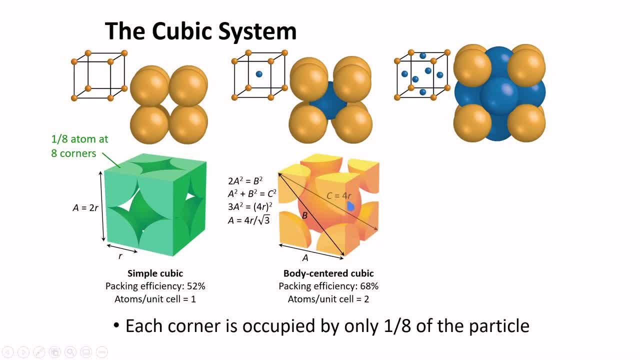 C is equal to 2a squared, then C squared can be calculated. C is equal to 2a squared to 4r, Hence A is equal to 4r over square root of 3.. Phase-centered cubic has the highest packing efficiency of the three, around 74% There. 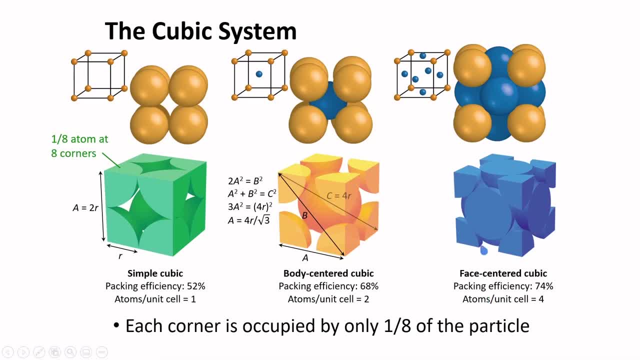 are four atoms per unit cells. The three atoms comes from the atoms on the side of each phases and the fourth atom comes from the combination of the 1-8th particles on each corner. If the length of the side is known, then we can easily determine the length of the diagonal. 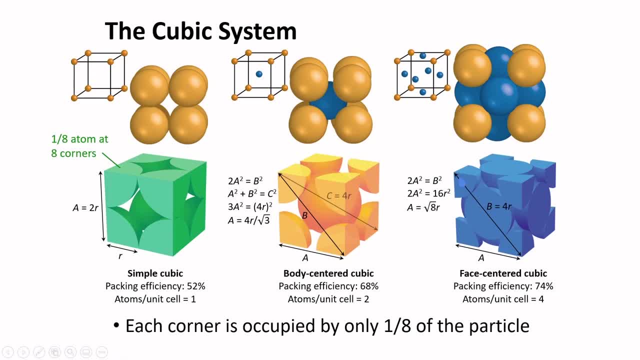 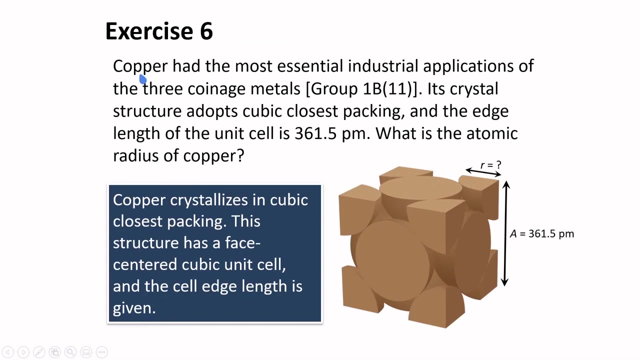 of one phase. by Pythagorean theorem, If B is equal to 4r, then B squared is equal to 16r squared. Hence A is equal to the square root of 8r. Exercise 6. Copper has the most essential industrial application of the three coinage. 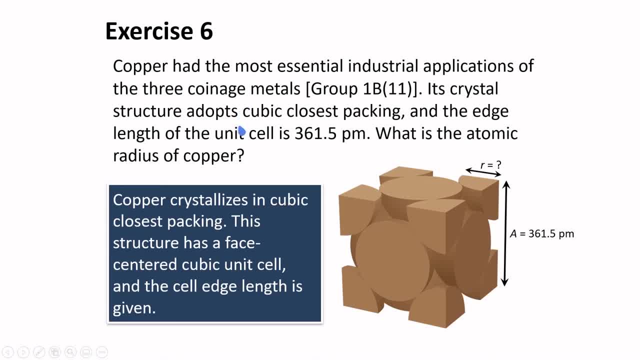 metals. Its crystal structure adapts cubic closest packing and the edge length of the unit cell is 361.5 km. What is the atomic radius of copper? Given that copper has a cubic closest packing, then we can use the formula given in the previous. 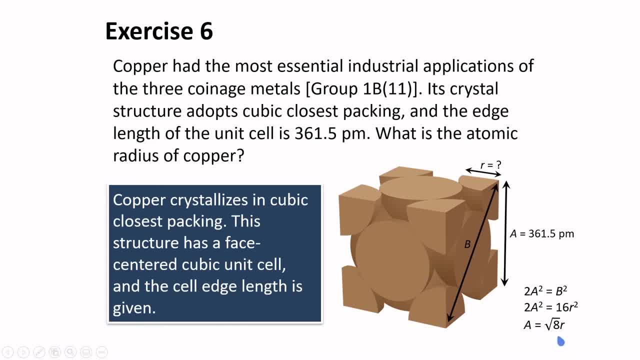 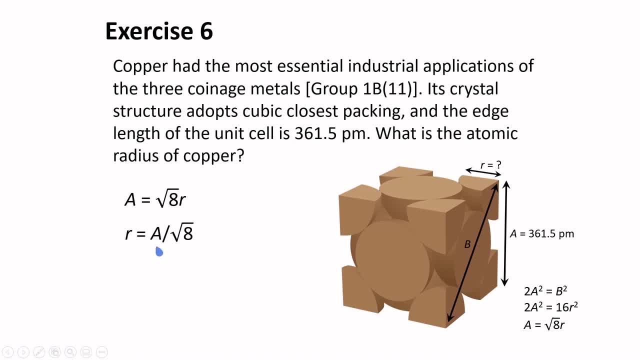 slide. A is equal to 3r. What is the atomic radius of copper? Given that copper has a cubic closest packing, then we can use the formula given in the previous slide: square root of 8, R. Rearranging the equation will result in R being equal to A over square. 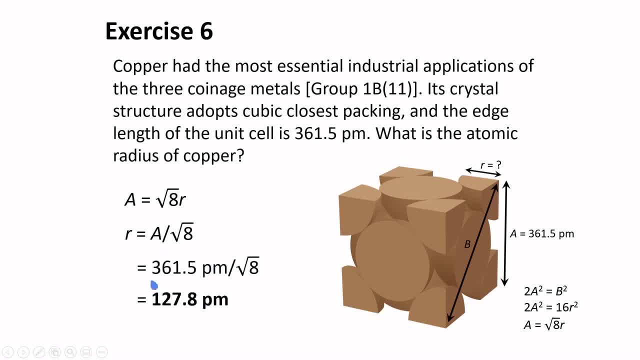 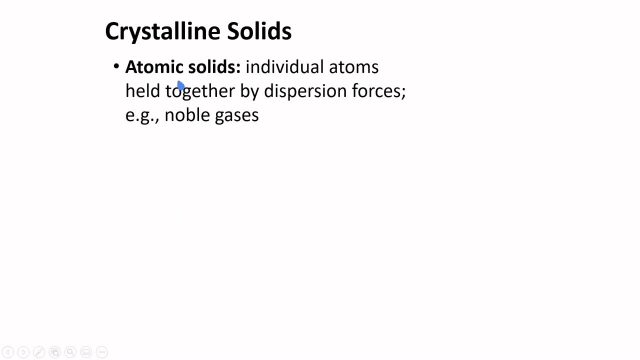 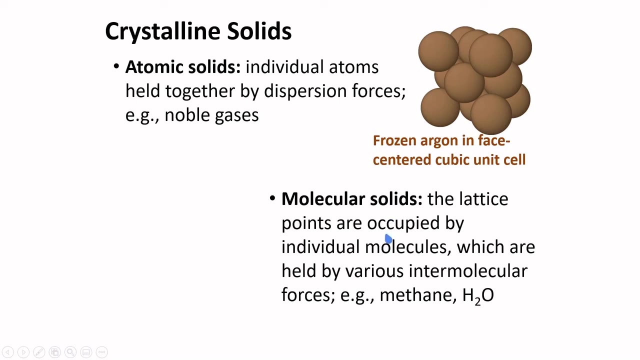 root of 8, which gives the radius equal to 127.8 decometers. In atomic solids, individual atoms are held together by dispersion forces, for example noble gases. Frozen argon exists in phase-centered cubic unit cells. In molecular solids, the lattice points are occupied by individual molecules which are 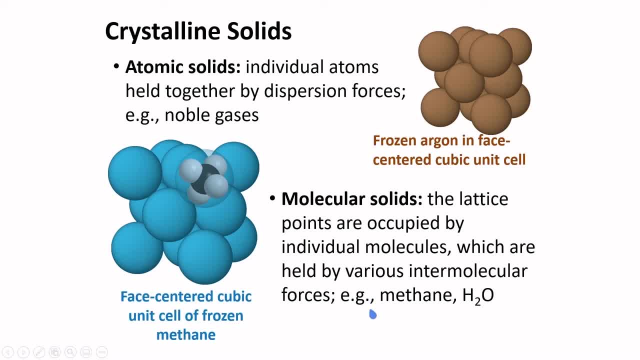 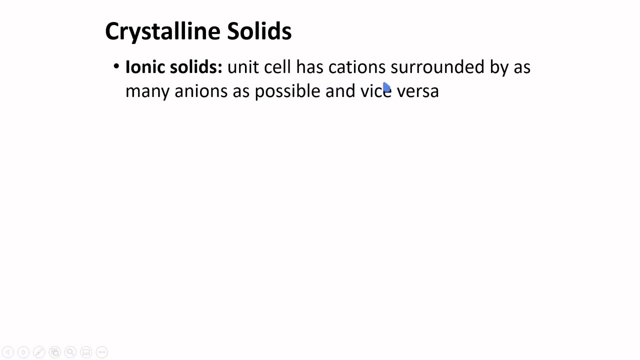 held by various intermolecular forces, for example, in this case here, Methane and water. Methane exists in phase-centered cubic unit cells, In ionic solids unit cell has cations surrounded by as many anions as possible, and vice versa. 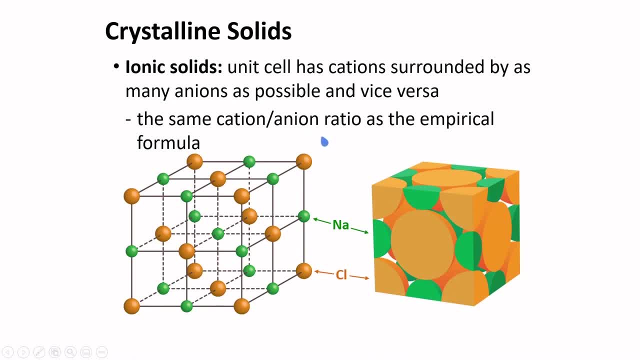 It has the same cation to anion ratio as the empirical formula. In ionic solids unit cell has cations surrounded by as many anions as possible, and vice versa. In ionic solids unit cell has cations surrounded by as many anions as possible, and vice versa.